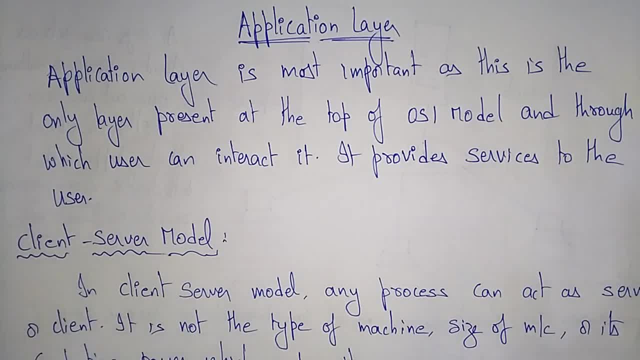 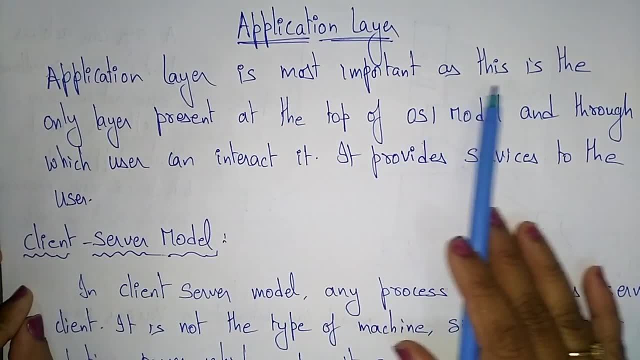 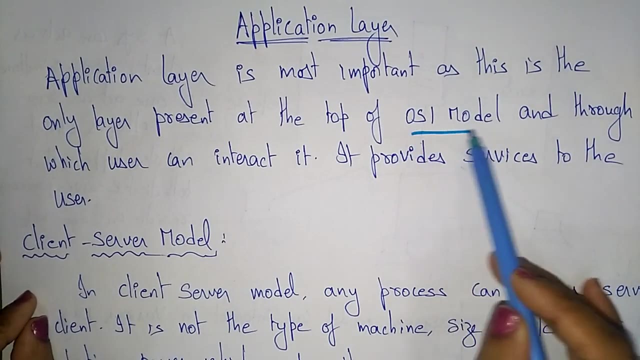 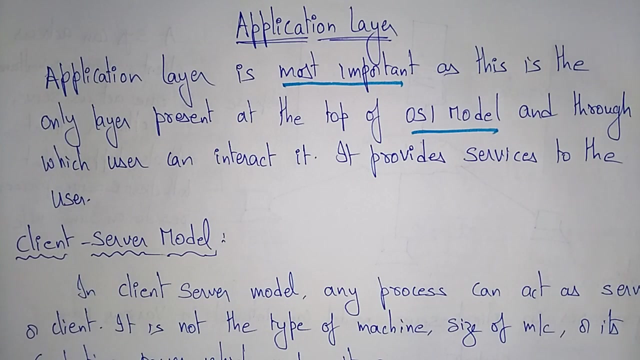 Now let's see the application layer, how the data communication will be established in the application layer. Application layer is the most important, as this is the because, as this is the only layer present at the top of the OSI model, Application layer is the most important. Why we call it as a most important? because it is the only layer present at the top of the OSI model and through which users 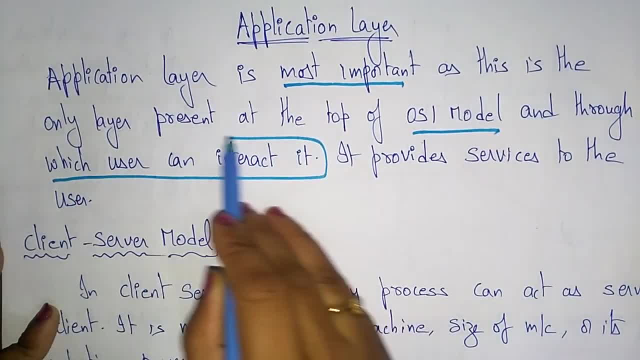 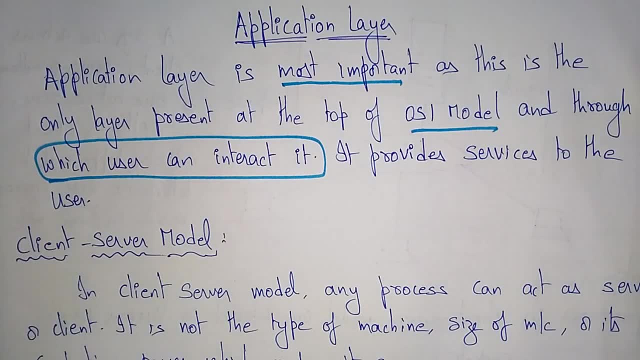 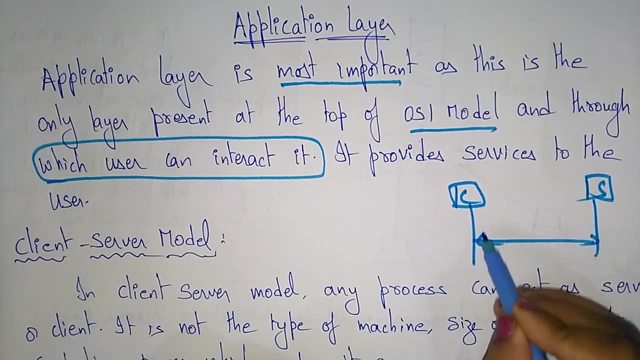 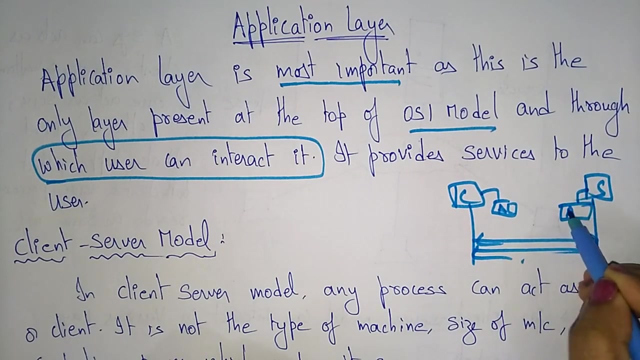 can interact it. Main thing is the user is going to interact with the system with the help of the application layer, because it is the topmost of the OSI model. So, whatever the system you are taking, the client and the server. if you want to make a communications between the client and the server, the first it has to interact with the application layer, and here also the server has to interact with the application layer. Okay, here the client and servers are nothing but the user. 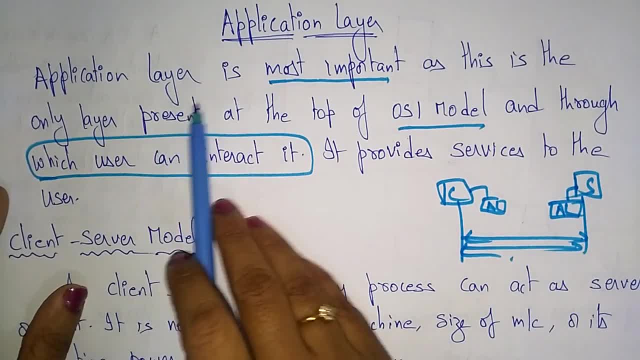 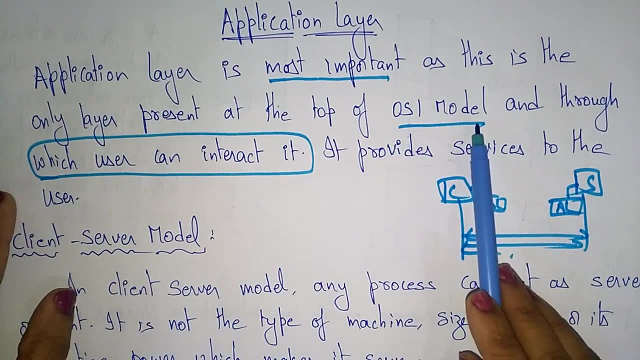 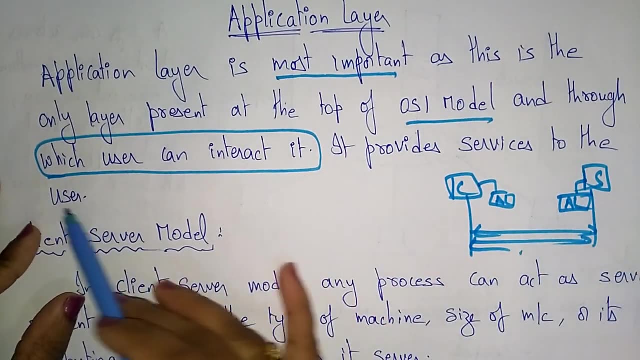 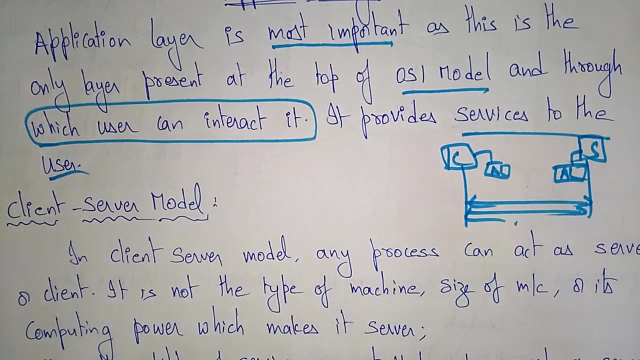 Let's take this of the users. Application layer is the most important as this is the only one layer, only layer present at the top of the OSI model and through which user can interact. it It provides service to the user. The main thing of application layer: it is providing service to the user. Let's take one of the example for the application layer, that is a client server model. The client server model is one of the application for the user. 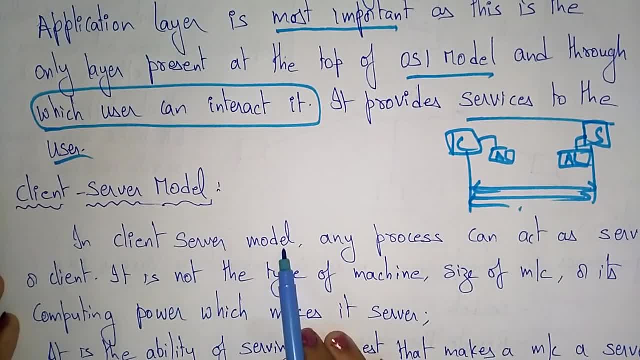 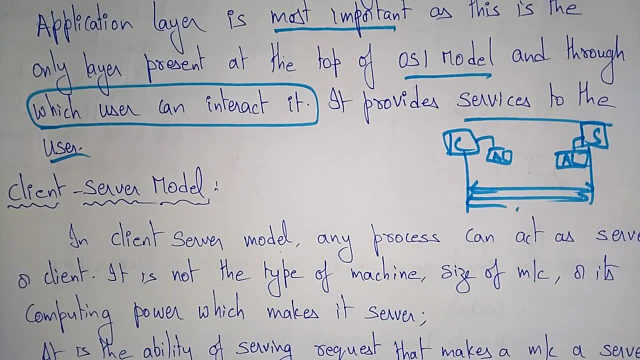 Application layer. In client server model any process can act as a server or a client. Okay, either this side or that side. So I'm one time I'm act as a server, Next time I may act as a client. Suppose I'm suppose I'm interacting with you students, I'm the server and you are the clients. Okay, suppose, if I'm interacting to my teacher and I'm the client, and my teacher was a server like that. So in client server model I'm the client. 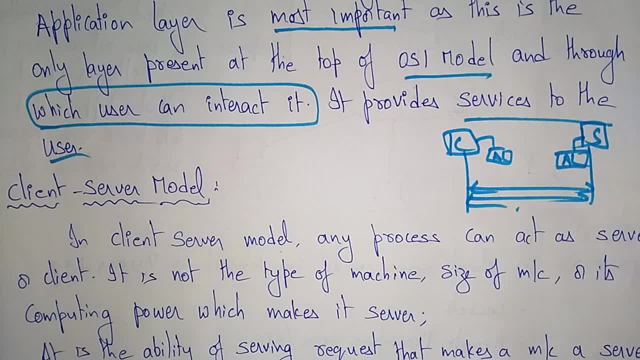 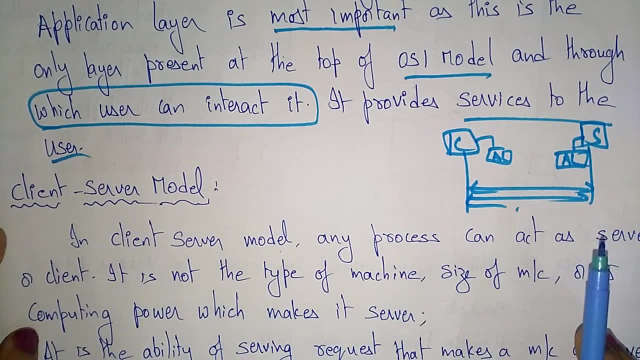 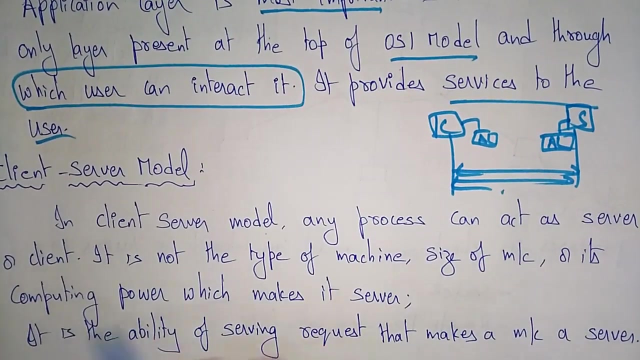 It is not the type of the machine and the size of the machine or its computing power which make it server. Okay, this point. you have to be remembered that it is not the type of the machine, whatever the client system you are taking, whatever the server system you are taking, It is we are not talking about the type of the machine and the size of the machine or its computing power which makes it server. It is the ability of the server. 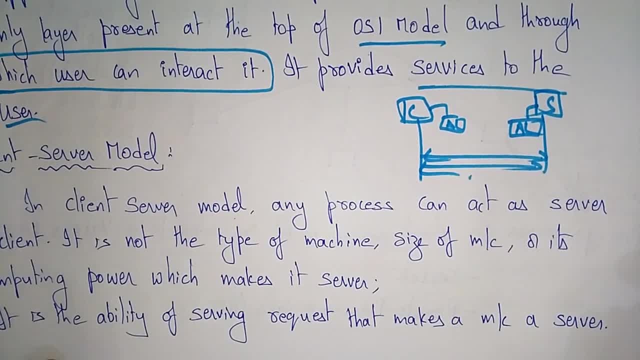 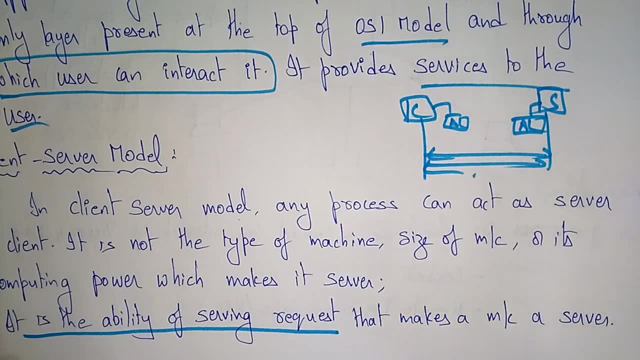 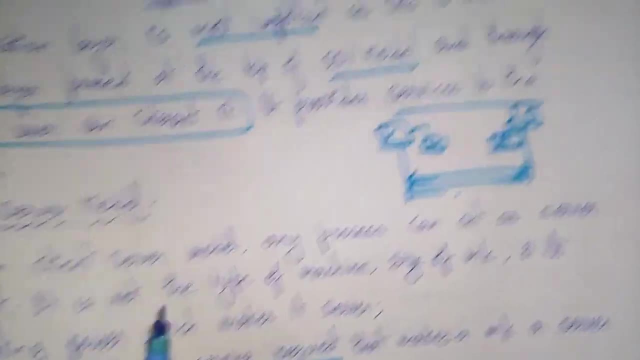 serving request. that makes a machine a server. so that is the thing. it is, the we are talking about the ability of the serving request. which which system is having the ability of the serving request? that makes as a machine a server, not the type of the machine and the size of the machine. 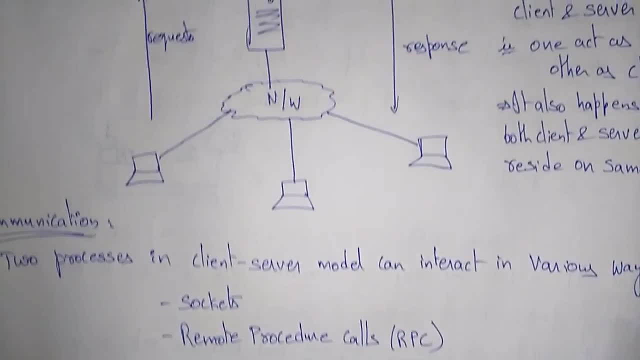 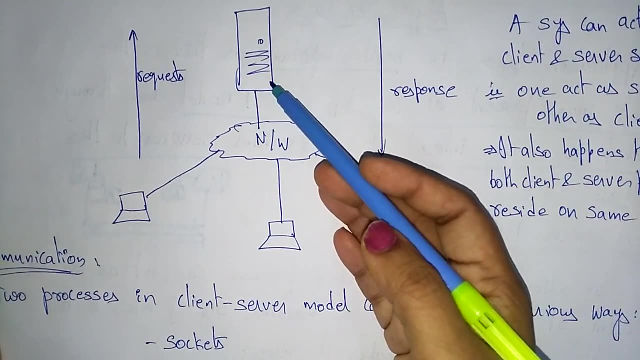 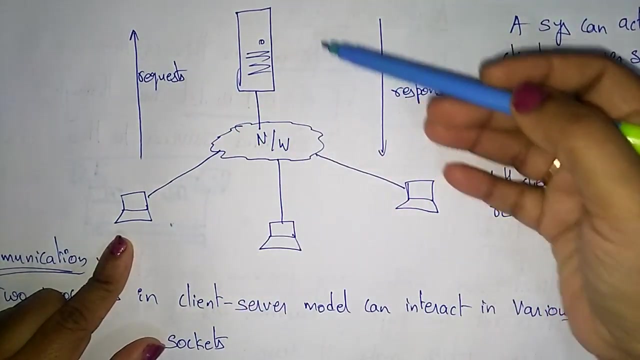 okay, so see here the client server model. uh, here let's take a system. any server- or it sometimes server- acts as a server and it acts as a client. here the systems are there, all connected in the network. here it is requesting and the server is giving the response. a system can acts as a client. 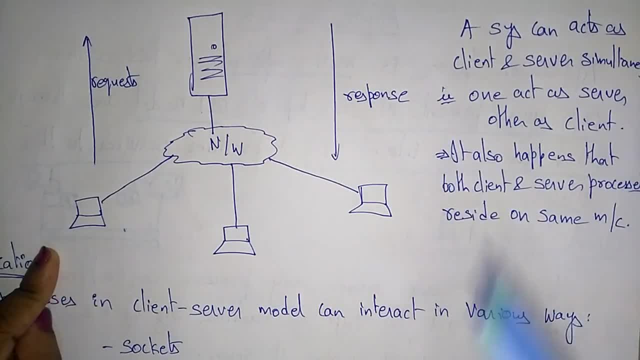 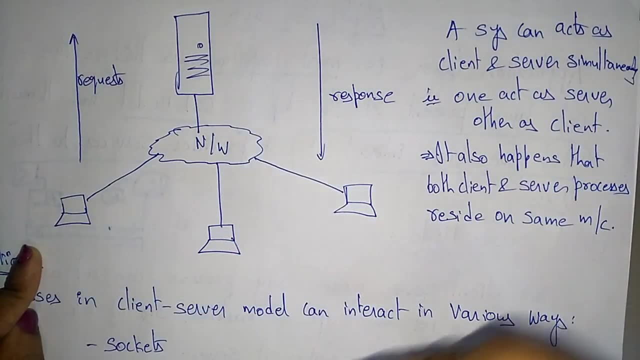 and server simultaneously. how can a system can access a client and server simultaneously, that is, one system can act as a server and other system as a client. this time, next time the other system act as a client and next system access server. they are acting client server simultaneously. 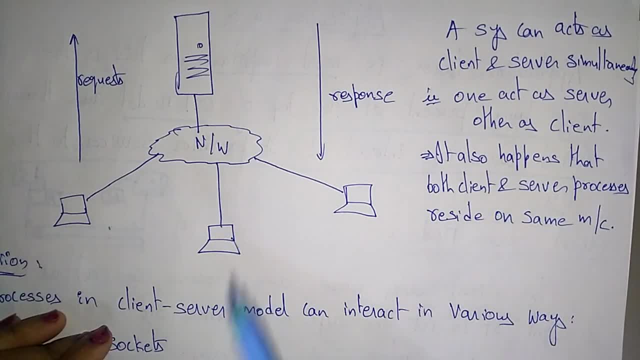 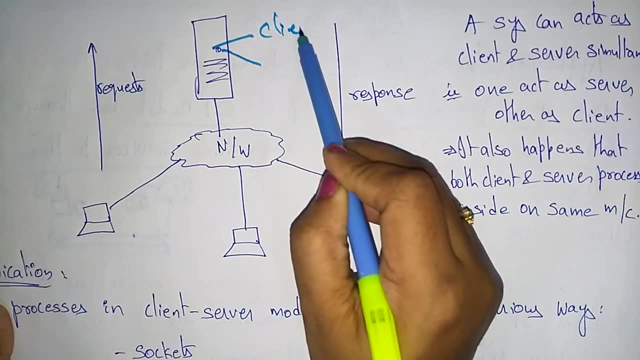 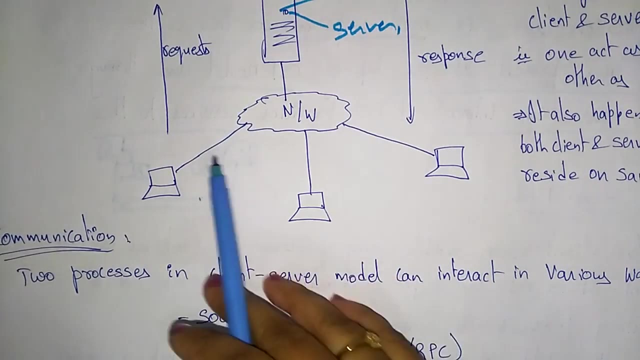 they are acting client server simultaneously. they are acting client server simultaneously. it also happens that both client and server process resides on a same machine. there may be a chance in the single machine both the client and servers may be present. okay, it may happen. let's see the communication. so, whatever the communication that is going to, 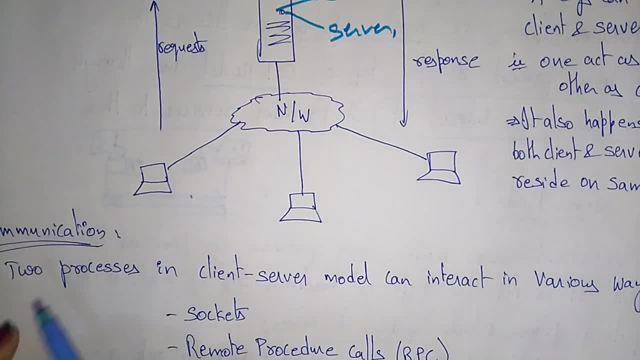 be established in the application layer. there is two process in client server model cut interact with various ways. one is a socket and another remote processor call with the application layer. there is two process in client server model cut interact with various ways. one is a socket and another remote processor. call with the help of these two process a 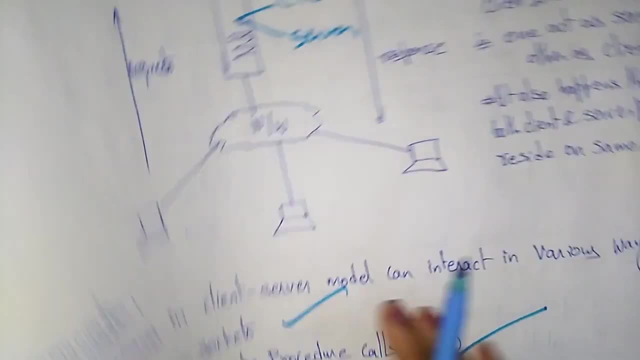 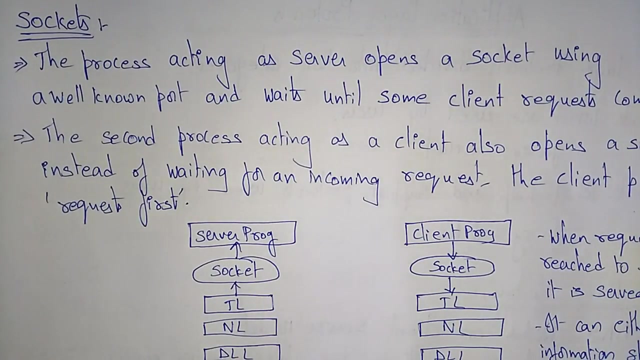 with the help of these two process, a communication will be established in the client server model. so what is the socket interface? now let's see the sockets. you all know socket a general. it's a wire cable. a socket is going to be connected to the point one of the plug point a socket is connecting.